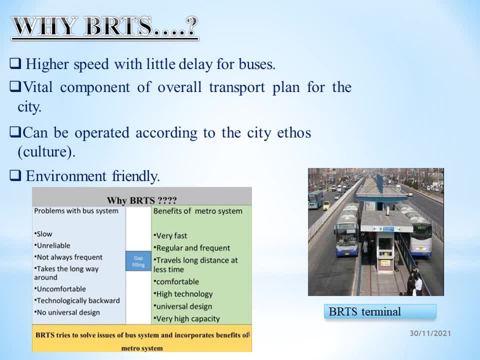 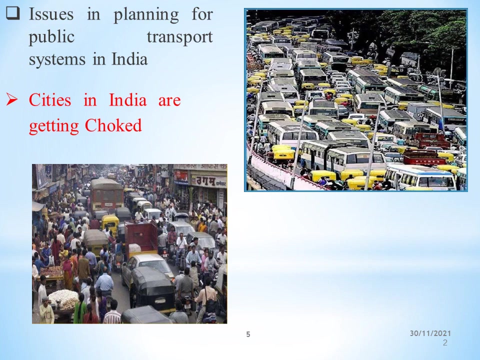 Now, why BRTS? Because higher speed with a little delay for buses, a vital component of overall transport plan for the city- Can be operated according to the city ethios, Also environmental friendly. Now issue in planning for public transport system in India. 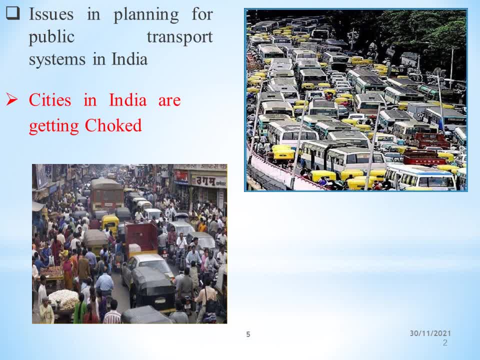 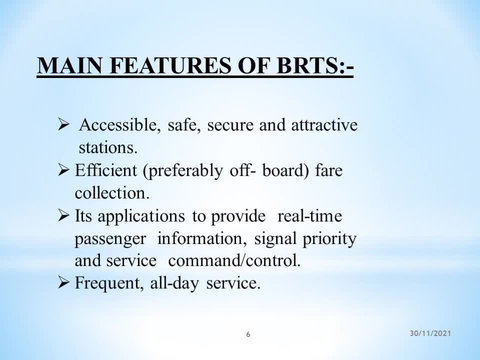 As we look into the pics, cities in India are getting choked due to unmanaged way of transportation. Main features, Features of BRTS: Accessible, safe, secure and attractive stations. Efficient fare collection. Its application to provide real-time passenger information. signal priority and service command. 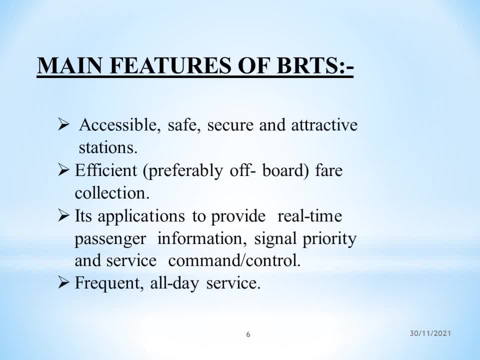 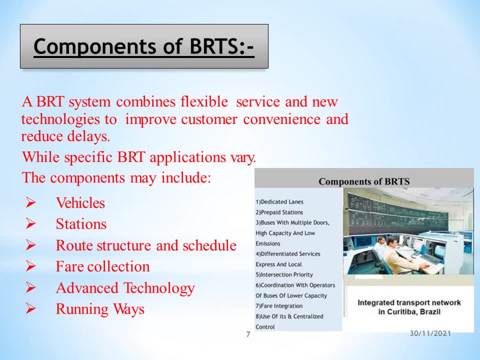 Frequent, ie all-day service is easily available. Now moving towards the components of BRTS. A BRT system combines flexible service and new technologies. Flexible service and new technologies to improve customer convenience and reduce delays. While specific BRT application varies, the components may include vehicles, stations, route structure and schedule, fare collection, advanced technology, running ways. 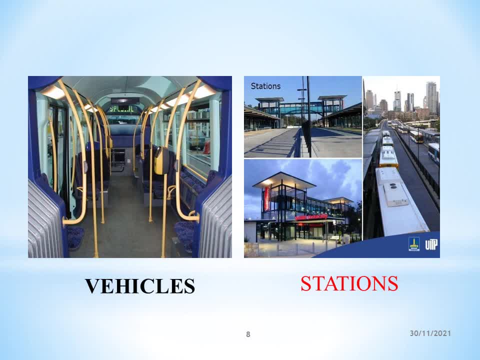 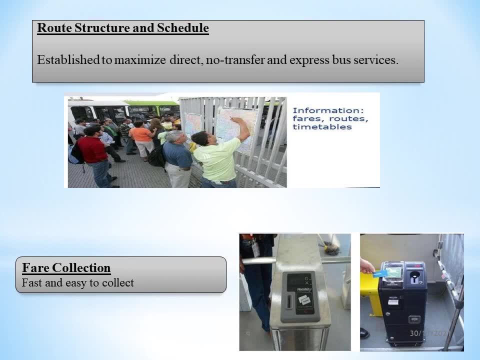 As we can see in the pics. Vehicles are there, Stations are there, Route structure and schedule established to maximize direct, no-transfer and express bus services. Fare collection is fast and easy to collect. Now, types of running ways. First, separate running way. 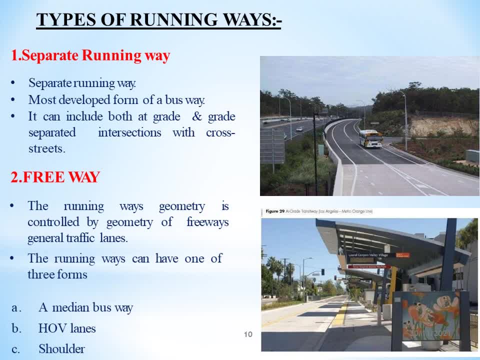 Separate running way, most developed form of a bus way. It can include both ad-grade and grade-separated intersections with cross streets. Second is freeway. The running way's geometry is controlled by geometry of freeway's general traffic lanes. A running way can have one of three forms. 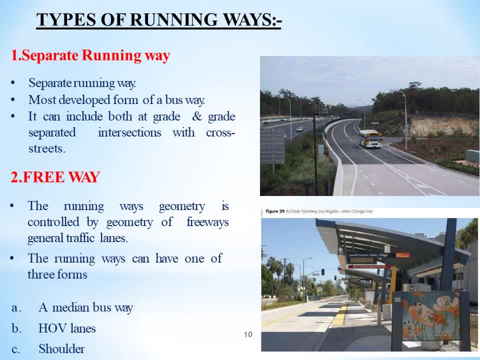 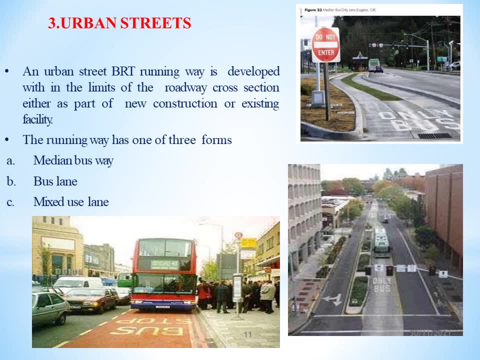 A median bus way, HOV lanes and shoulder Urban streets. An urban street BRT running way is developed within the limits of the roadway cross-section, either as part of new construction or existing. The running way has one of three forms: Mean bus way, bus lane, mixed-use lane. 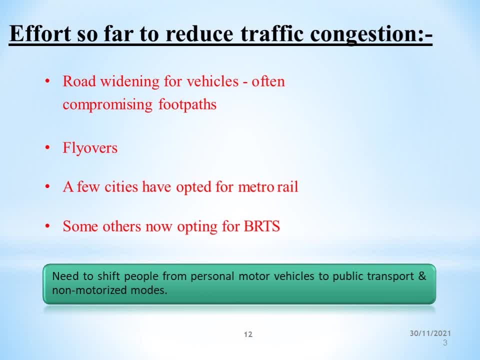 Now efforts so far to reduce traffic congestion, Road widening for vehicles, often compromising for footpaths, Flyovers. Cities have opted for metro, rail, Some others now opting for BRTs. Now need to shift people from personal motor vehicles to public transport and non-motorized modes. 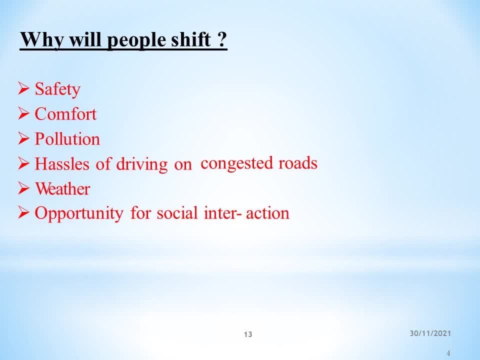 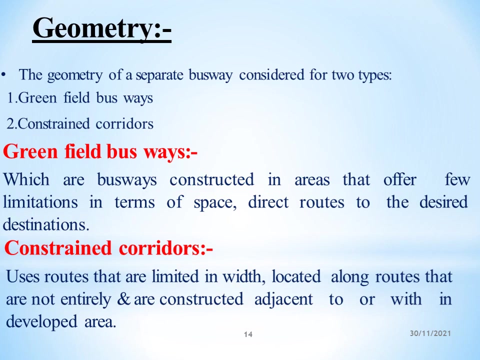 Why will people shift? Because of safety, comfort, pollution, hassles of driving on congested roads, weather, opportunity for social interaction. Moving towards the next slide, Begin with the geometry. The geometry of a separate busway, considered for two types. 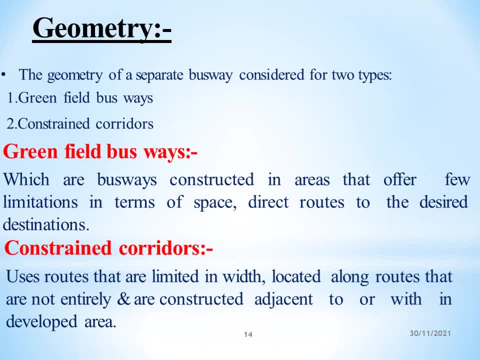 Greenfield busways- Constrained corridors. What is greenfield busways? Which are busways constructed in areas that offer few limitations in terms of space. direct routes to the desired destinations. Constrained corridors Uses routes that are limited in width, located along routes that are not entirely, and are constructed adjacent to or within busways. 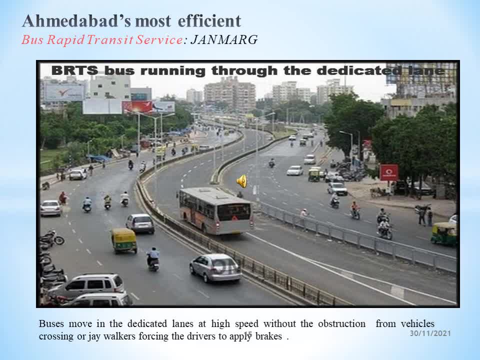 In the developed area. As we can see in the pic, it is Ahmedabad's most efficient bus rapid transit service, Known as JANMARG. Buses moves in the dedicated lanes at high speed without the obstructions from vehicle crossing or jaywalkers forcing the drivers to apply brakes. 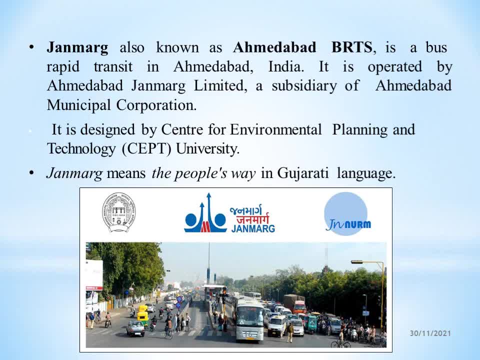 JANMARG, also known as Ahmedabad BRTs, is a bus rapid transit in Ahmedabad, India. It is operated by JANMARG Limited, a subsidiary of Ahmedabad Municipal Corporation. It is designed by Centre for Environmental Planning and Technology. JANMARG means the people's way in Gujarati language. Now, what is their background? Ahmedabad has a population of 5.7 million, which is likely to be 11 million by 2035.. This would lead to agglomeration of surrounding settlements like Naroda, which increases the area of the city by 1000 km2 by 2035.. 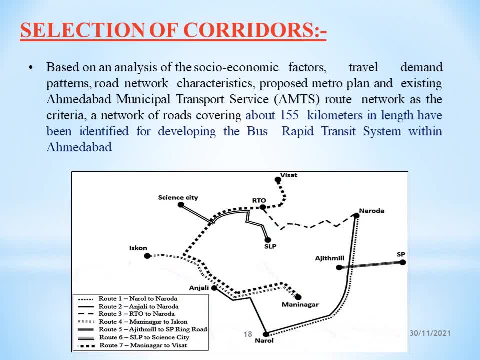 Ahmedabad has limited public transport. Now, the selection of the corridors Based on an analysis of the socio-economic factors- travel demand pattern, road network characterization, proposed metro plan and existing Ahmedabad Municipal Transport Service Route network as the criteria, A network of roads covering about 155 km in length have been identified for developing the bus rapid transit system within Ahmedabad. 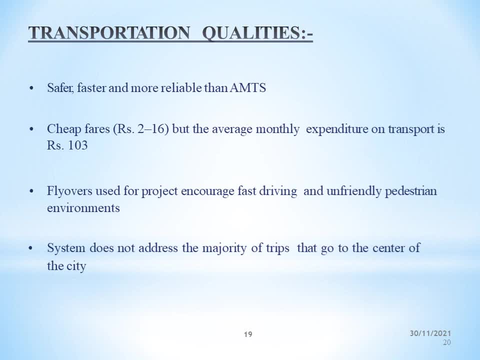 Transportation qualities Safer, faster and more reliable than AMTS Cheap fares. but average monthly expenditure on transport is Rs.103.. Flyovers used for projects encourage fast driving and unfriendly pedestrian environments. System does not address the majority of trips that go to the centre of the city. 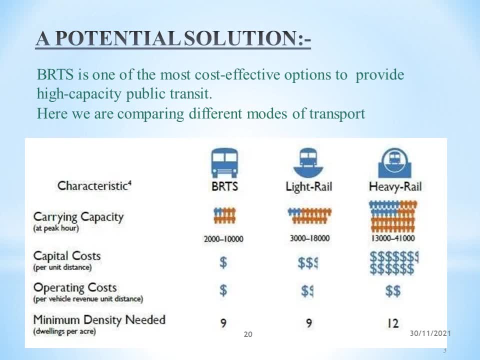 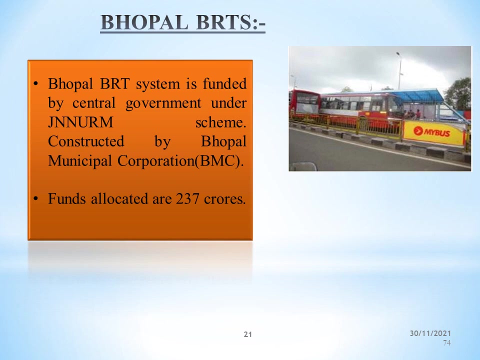 A potential solution. BRTS is one of the most cost-effective options to provide high-capacity public transit. Here we are comparing different modes of transport like BRTS, light rail and heavy rail Bhopal. BRTS- Bhopal BRT system is funded by central government under JNNURM scheme. 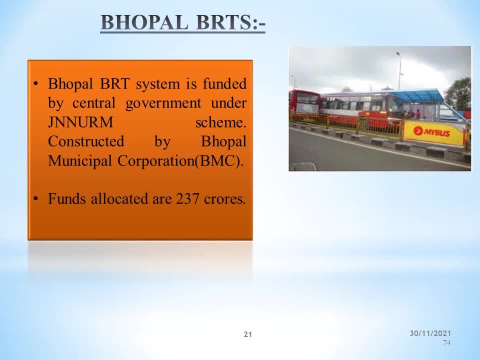 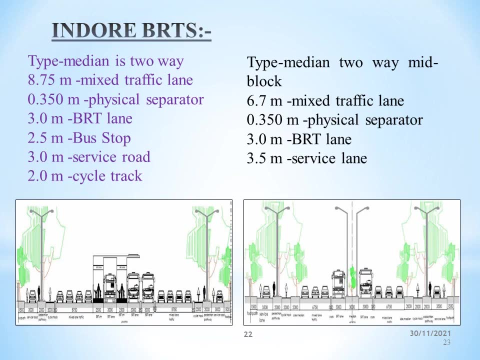 constructed by Bhopal Municipal Corporation. Funds allocated are Rs.237 crores. Indore BRTS Type median is two-way In this: 8.75 m mixed traffic lane, 0.350 m physical separator, 3 m BRT lane, 2.5 m bus stop, 3 m service road, 2 m cycle track. 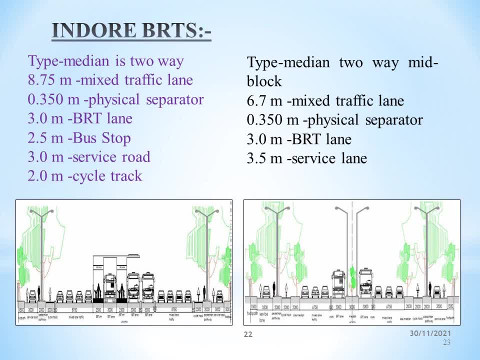 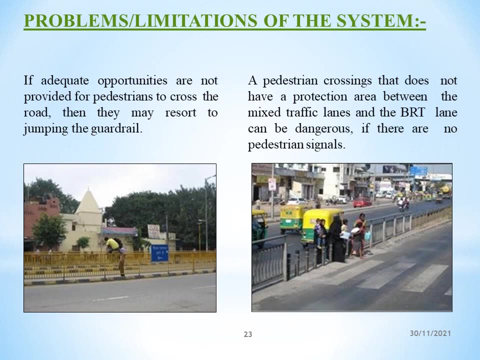 Type: median: 2-way mid-block 6.7 m mixed traffic lane. 0.350 m physical separator. 3 m BRT lane, 3.5 m service lane. Now problems or limitations of the system: If adequate opportunities are not provided for pedestrians to cross the road, then they may resort to dumping the guardrail. 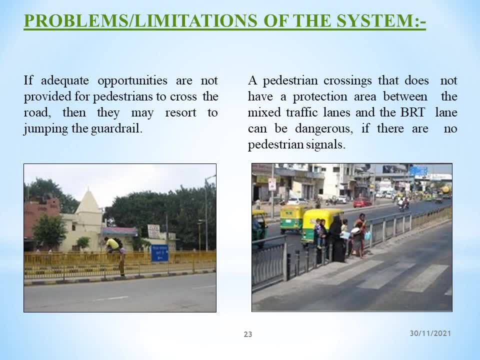 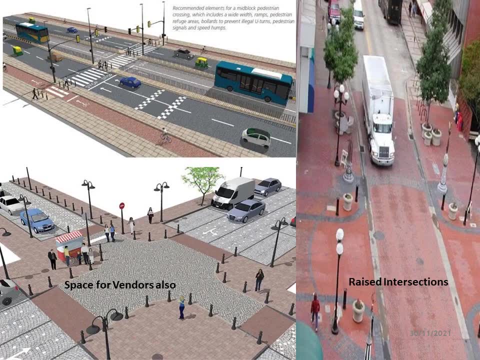 A pedestrian crossing that does not have a protection area between the mixed traffic lane and the guardrail. The BRT lane can be dangerous if there are no pedestrian signals. As we can see in the pic raised, intersections are there and space for vendors are also provided. 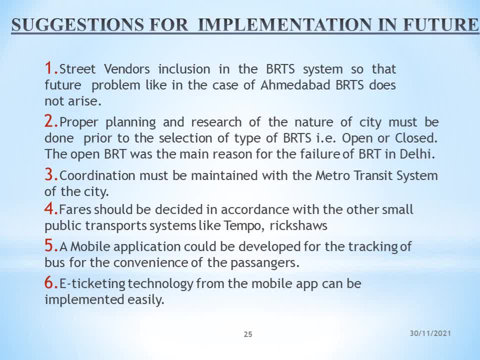 Now suggestions for the implementation in future Street vendors inclusion in the BRTS system. so that future problem like in the case of Ahmedabad BRTS does not arise. Proper planning and research of the nature of city must be done prior to the selection of type of BRTS that is, open or closed.